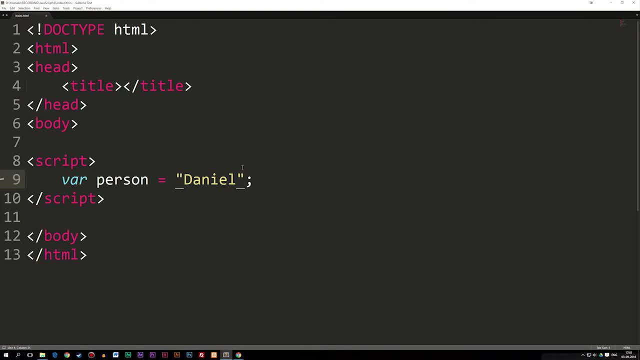 the double quotes, i can write some text. now, when you use double quotes, it's called a string and, as you guys can see- inside my editor at least, it turns yellow, which means that right now it's seen as plain text. now i can also go ahead and write a number in here if i want to, which is still going. 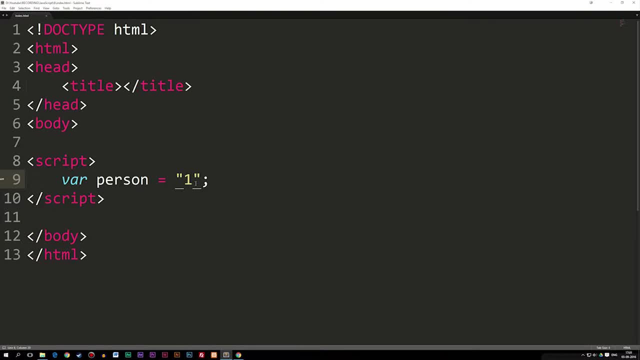 to be seen as number one, but the data type is a string. if i want to create a number data type, i'm just going to go ahead and write one or two or whatever. i want to write in here some kind of number, and this is going to make the browser see this as a number data type and not as a string. 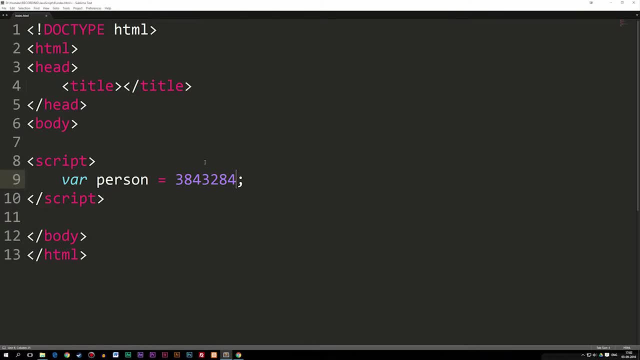 okay. um, the differences between using, you know, simple numbers or a string like so depends on what kind of function you're creating. so you might want to create a string at some point, or a number, so it depends on the purpose of the data type. so i'm just going to go ahead and 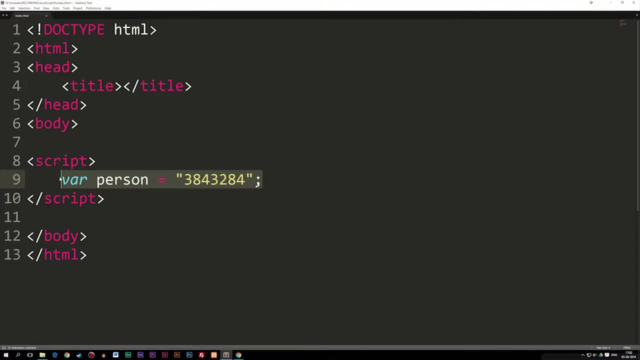 write the variable. so we're going to say, please, the variable is person, and then i'm going to write an array here and i'm going to go ahead and create an array and i'm going to write a variable which is a person that we're going to use for this purpose. now the third piece of data we're. 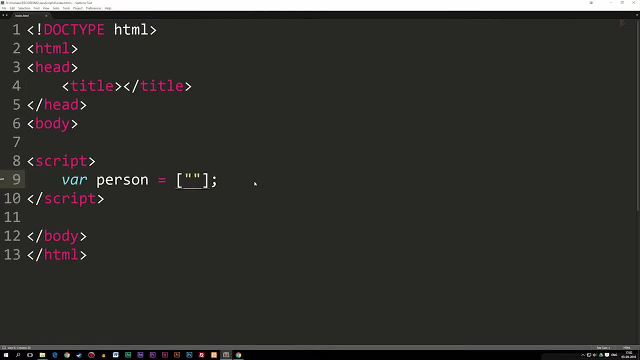 going to talk about is something called an array. so i can actually create an array by writing. let's actually go ahead and keep our variable person here. i can write: we create an array. we can store different types of information inside one variable. so right now i have daniel, i have lisa and i might have susie, which should be a string. there we go. 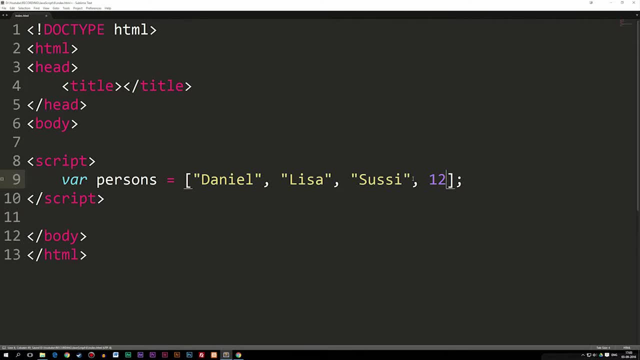 i could also store something called a number data type if i wanted to, without the quotation marks. now, basically, what this does is that it allows for us to create different types of data inside one variable, which can be useful for creating something like a loop which we haven't actually. 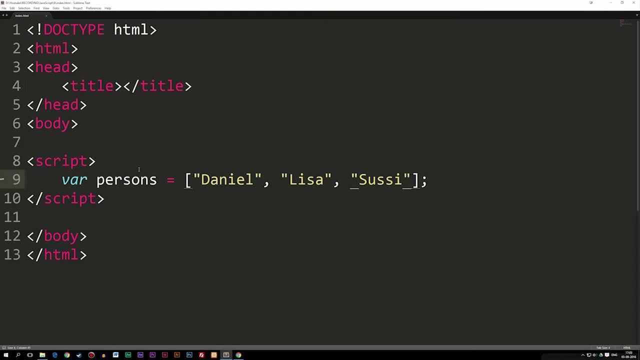 talked about yet, but later on you might want to store different data types. let's say you have a person who writes different types of information, you know more than one piece of information and submitting it to your website and you want to save it inside. you know a variable. then you can do. 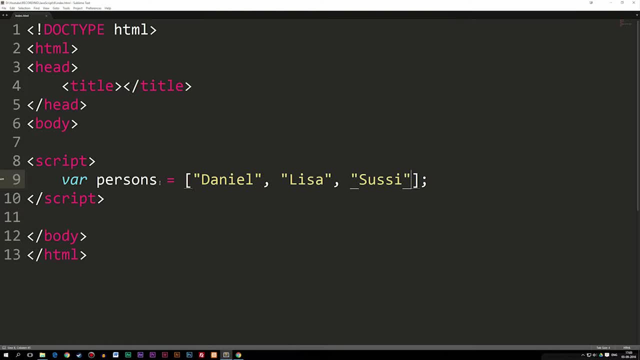 with this way to store many different types of information inside one variable, instead of having to create three different variables for each person, which is going to lessen your code and also be more useful for you. Now, the fourth data type we're going to talk about is something called an object. 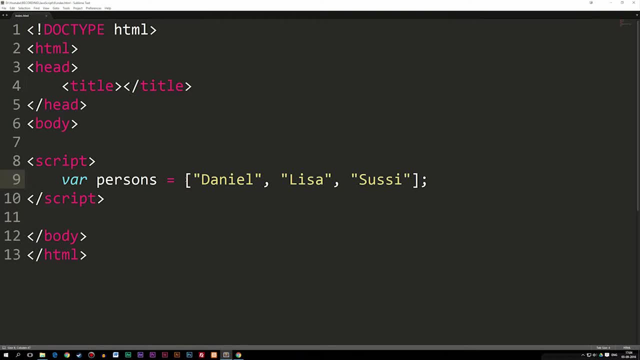 We're going to get more into objects later, but for now I just want to show you guys what an object is, so you guys have a basic understanding of it. And when it comes to objects, you can also store many information inside one variable. But the difference here is that we actually have 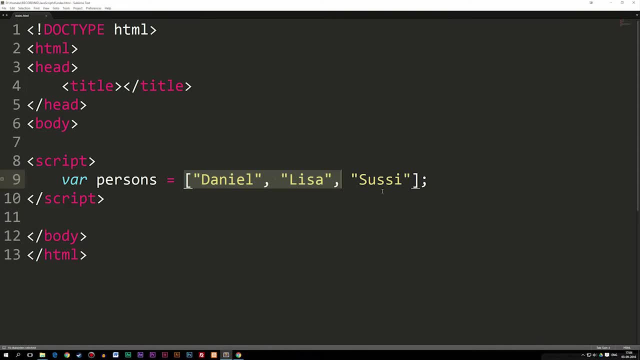 something called properties and a value. So if I want to go ahead and delete this array which was with the brackets, I can actually go and use curly brackets, open and close it, And inside the curly brackets we can start out by saying: okay, we have a person which is the object. So right now, 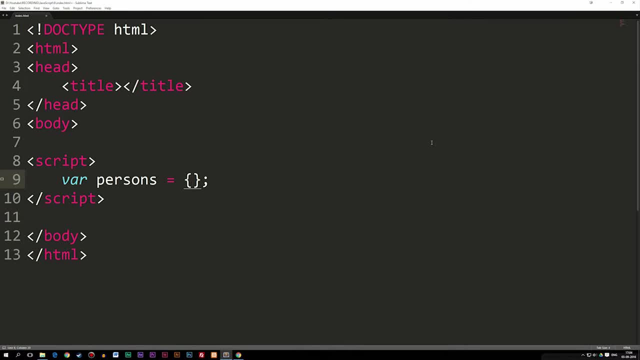 we're actually creating an object called persons, And well, that's actually changed. So let's say we have a person and this one person has different types of properties. Let's say it's me we're talking about. My name is. well, you should probably write name, which is the first. 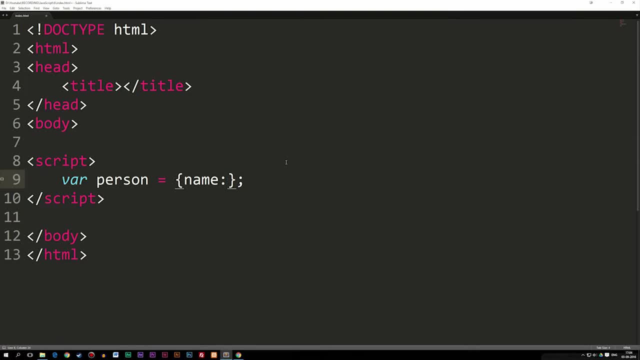 property and the value of my name is Daniel. Do you notice that I use the string, which is a data type, And after we have this one property, which is the name which is Daniel, because that's my name, I can write comma and say: 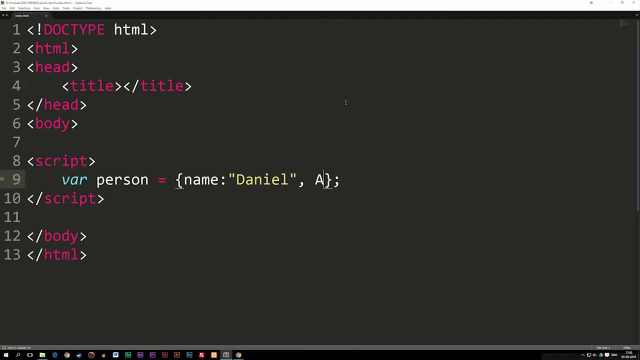 okay, another property of me could be my age, And that one could be equal to 25, because that's what I am right now. And then we can add another property which could be my- well, couldn't really be my height, because I don't actually know my height, But we could say number of legs, because I know I. 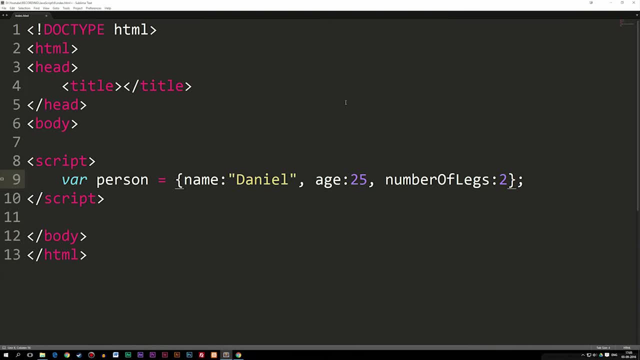 do actually have two legs. There we go, And this is a basic way we can store properties, and then we can use it to a object and actually have different, you know, have the properties equal to something, And this is something we're going to use a little bit later on when we have something.